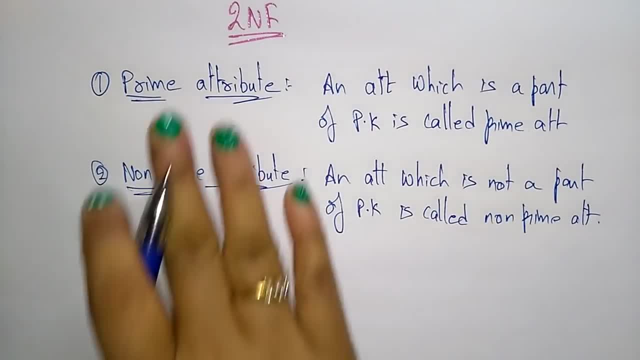 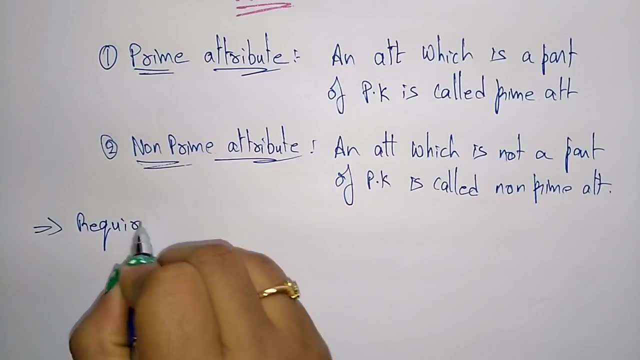 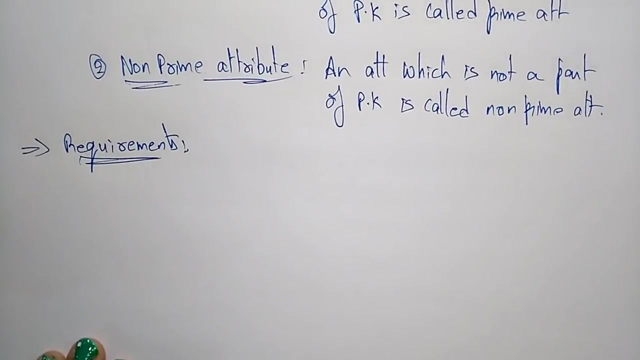 Okay, So let us know about these two concepts: prime attribute and non-prime attribute. Now let us see the requirements of 2NF. First see the requirements, Then we will see what is this 2NF is and how we decompose the 2NF. decompose 2NF table. 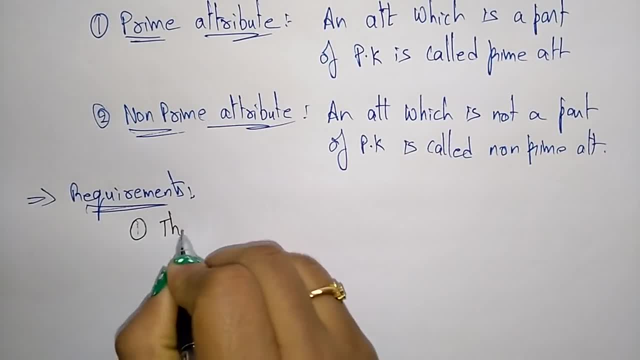 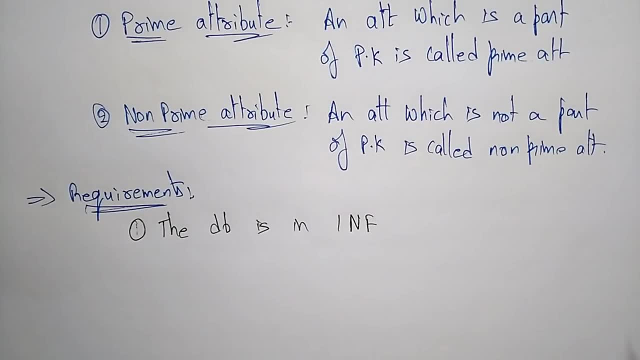 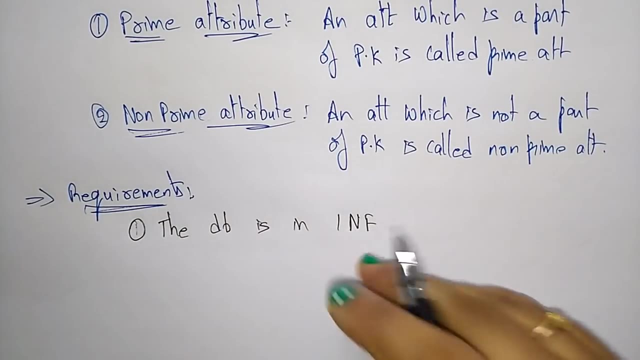 So requirements is: first, the database is in 1NF. The first step you have to follow is, whatever the database, whatever the table you have taken, that table should be in 1NF, Means it follow the 1NF requirements, like the table contains at least one primary key and all the values in the tables should be atomic. 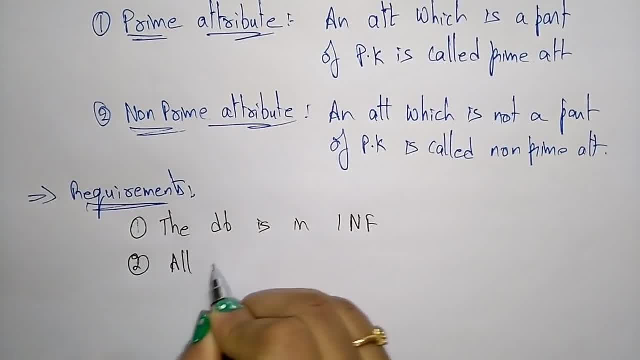 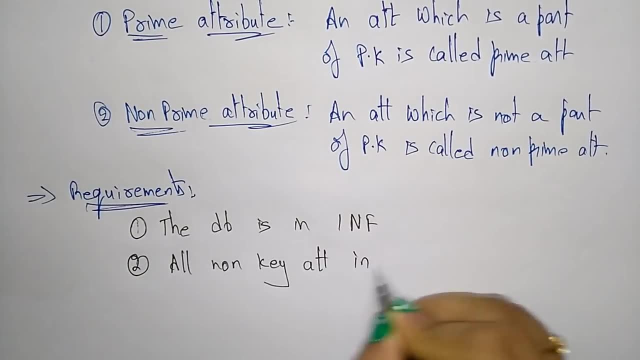 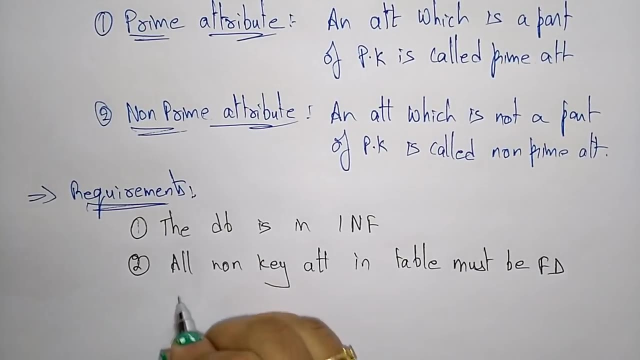 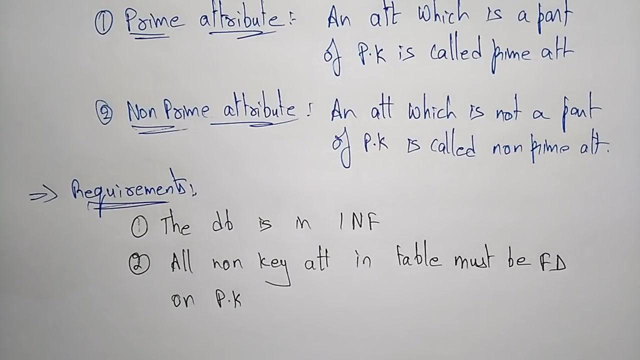 And the second is all non-key attributes. so non-key attributes means non-prime attributes. Non-key attributes in table must be functionally dependent on primary key. okay, So in 1NF you didn't. there is no condition that every attribute should be functionally dependent on the key attribute. 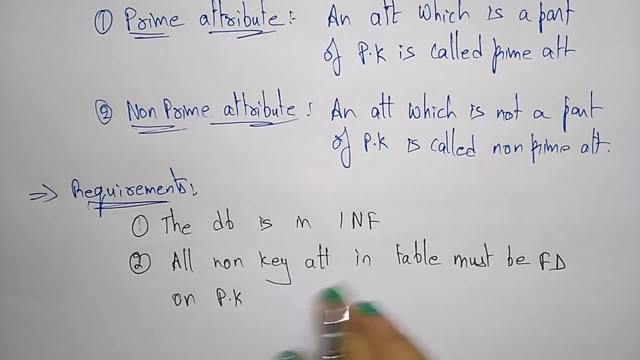 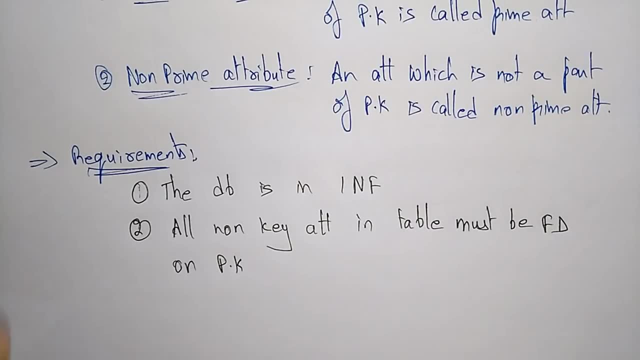 But in the 2NF all non-key attributes in table must be functionally dependent on primary key. So note that we have. we are only dealing with non-key attributes. So in this 2NF we are dealing with non-key attributes. 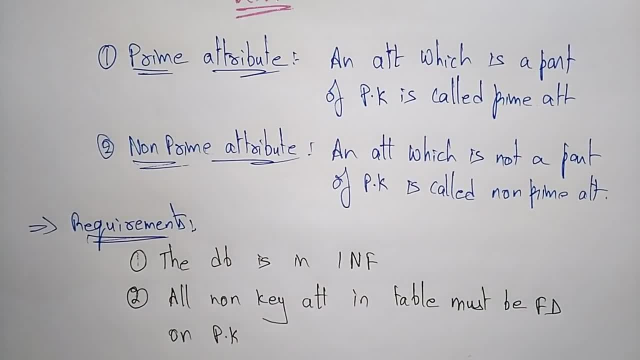 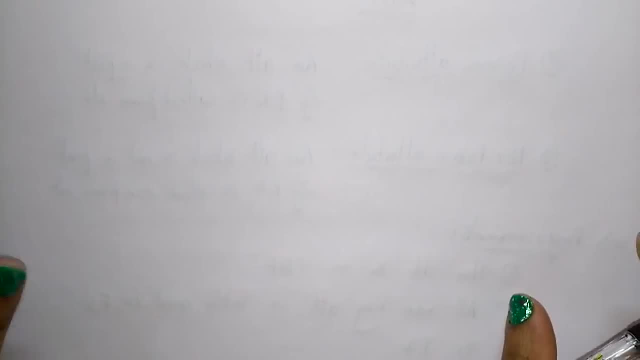 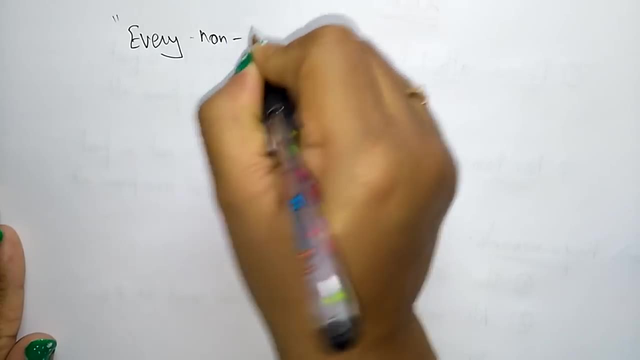 Those non-key attributes should always depends upon the primary key. So this is the requirements you have to follow. Now let us see the definition of this: 2NF. So what is the definition of 2NF? Every non-prime attribute. so I said, the non-prime attribute is nothing but. 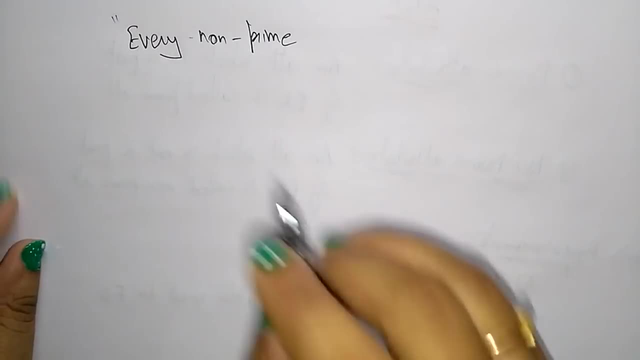 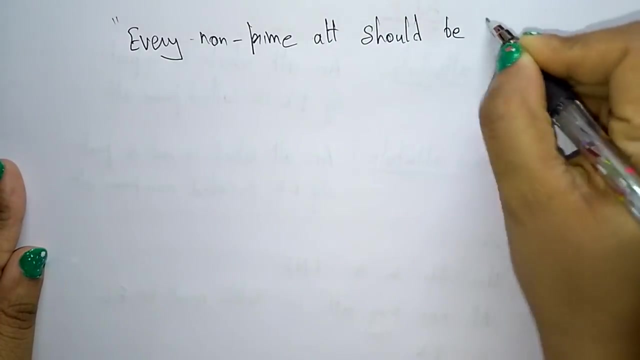 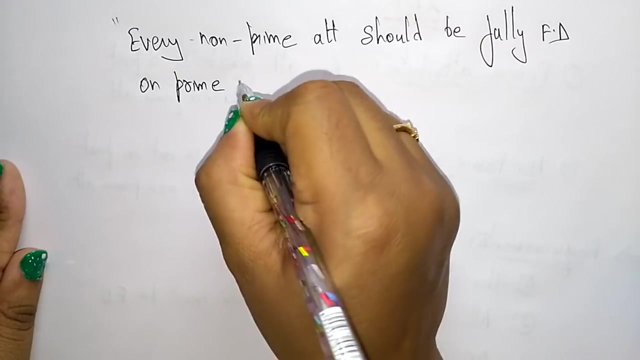 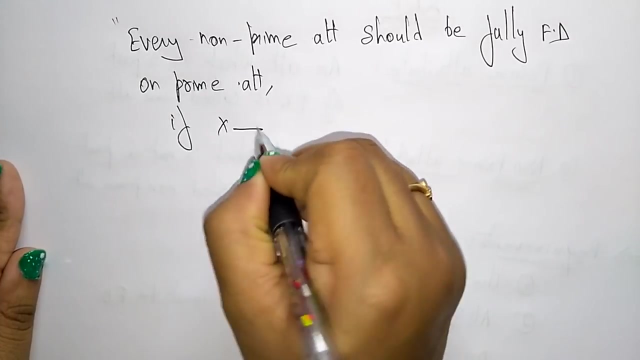 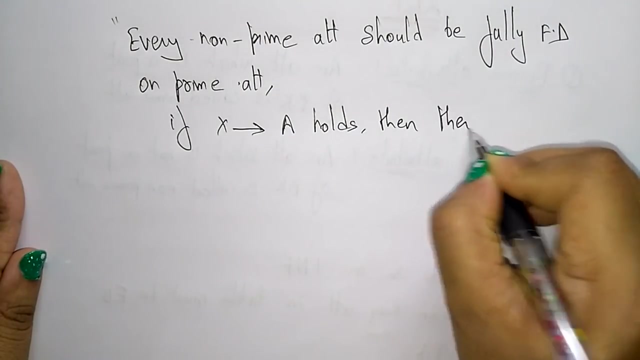 an attribute which is not a part of primary key, That is, non-prime attribute. Every non-prime attribute should be fully functional, dependent on prime attribute. if x determines a holds, then there should not be. 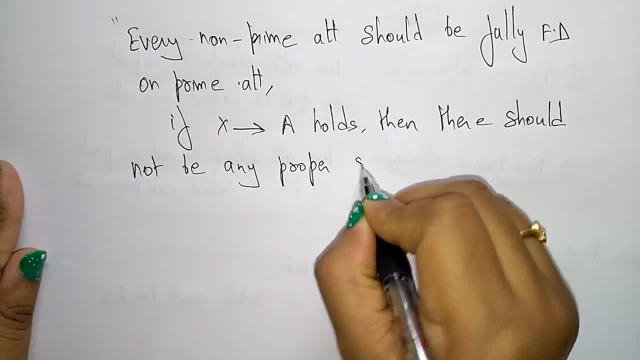 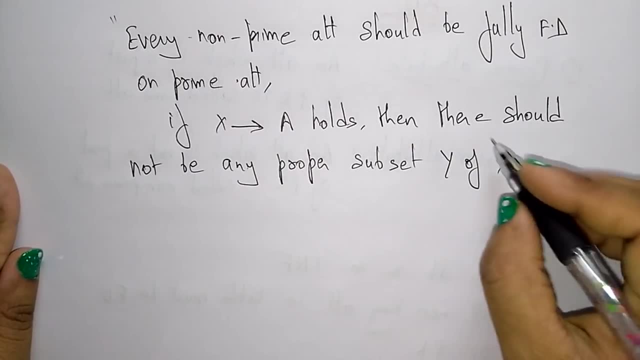 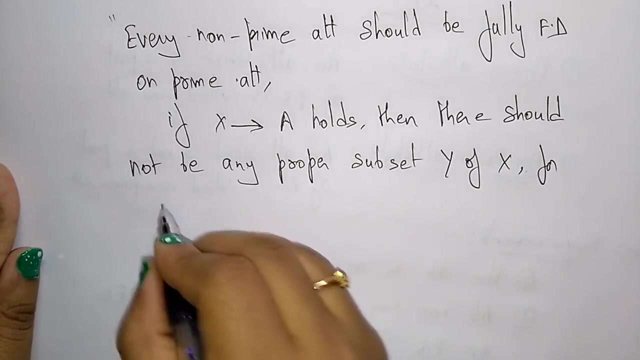 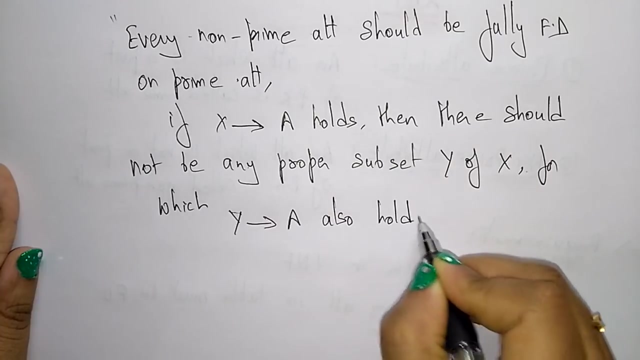 any proper subset. y of x means, just following the dependency relationship, functional dependence. Every non-key attribute should depends upon the primary key attribute, y of x, for which y determines a also holds true. Okay, So this is the definition of the 2NF. 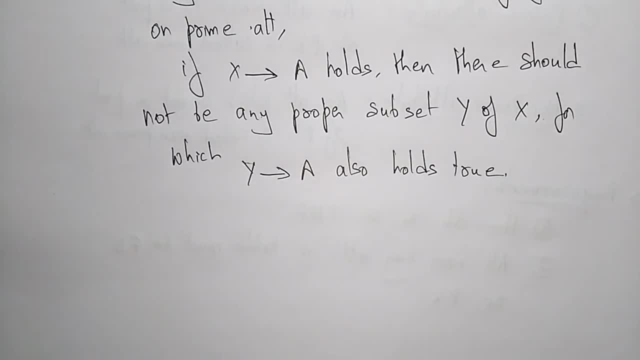 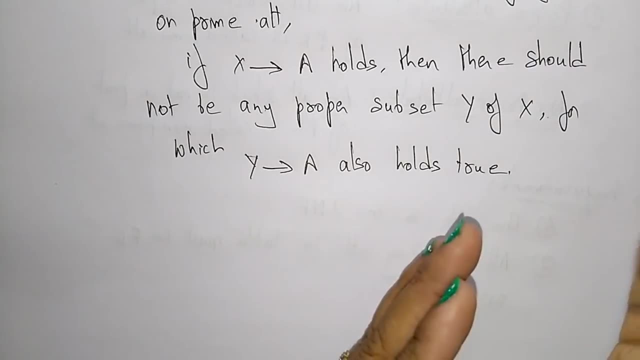 So here the redundant data across multiple rows of a table must be moved to separate table. So whenever you are having the redundant multiple rows of a table that should be moved to separate table means you are making to the new table. The resultant table must be related to each other by using some foreign key. 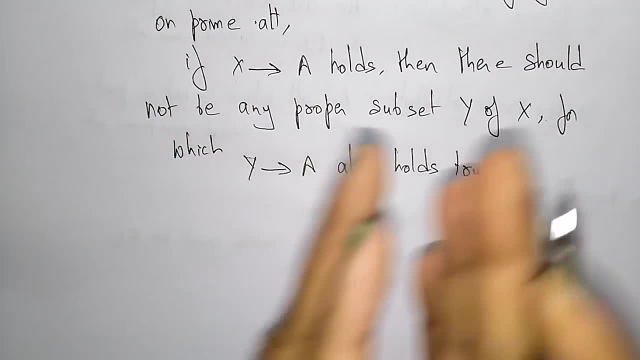 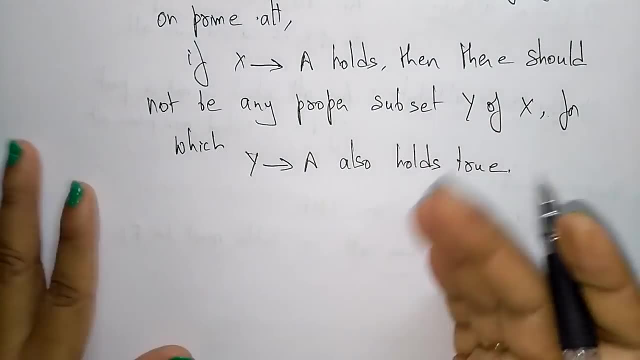 Means one table. you make it as a primary key in another table. If you are using that primary key is using in another table, then you make it as a foreign key. Okay, So that is about the rules You have to follow. means the requirements that you are needed for the 2NF. 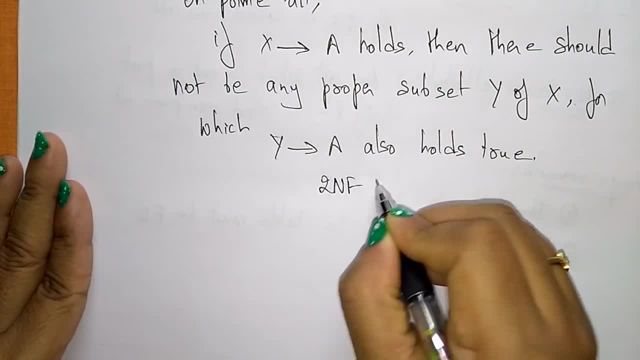 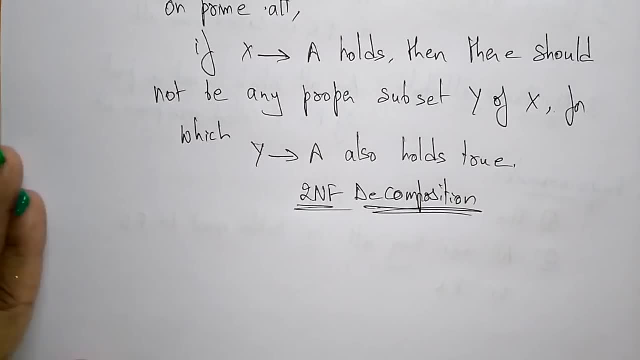 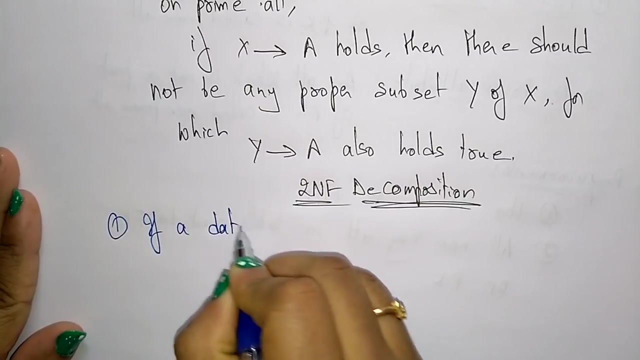 Now let us see the 2NF decomposition, How we decompose the 2NF, 2NF decomposition. So first is how. what is the first step you have to if a data item is fully functional dependent? 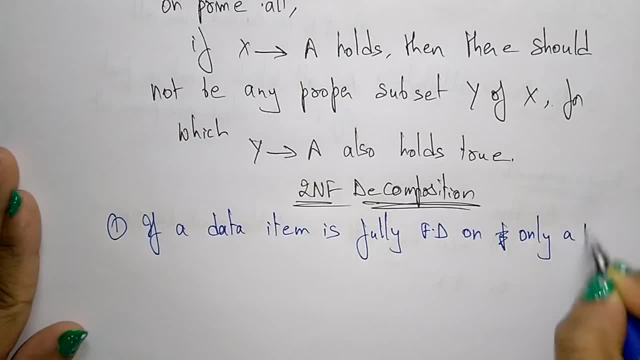 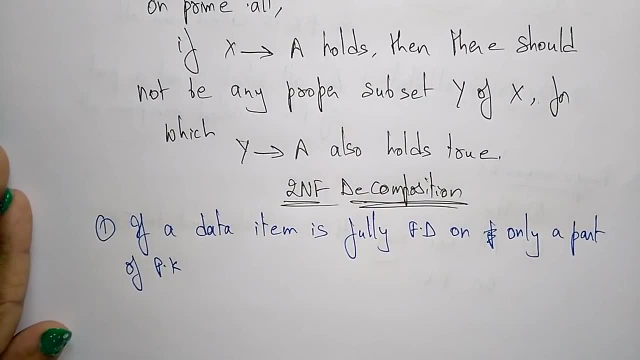 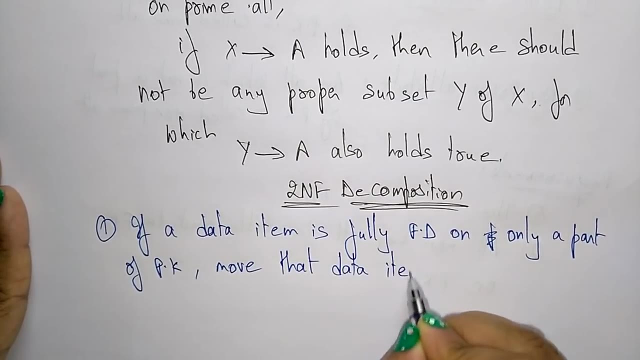 on only a part of primary key. So, whatever the data item you have taken that is fully functional, dependent on only part of a primary key, then move that data item and part of primary key to a new table. So this is the first step you have to follow while you are decomposing a relation into 2NF. 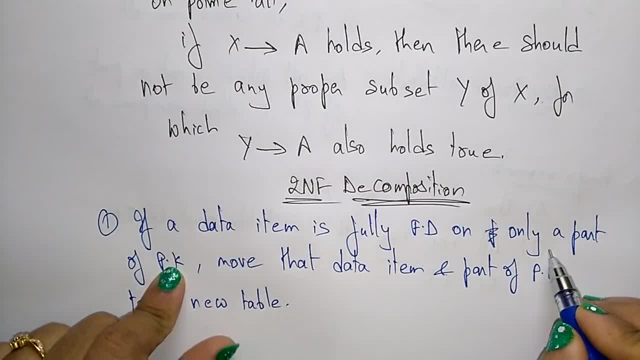 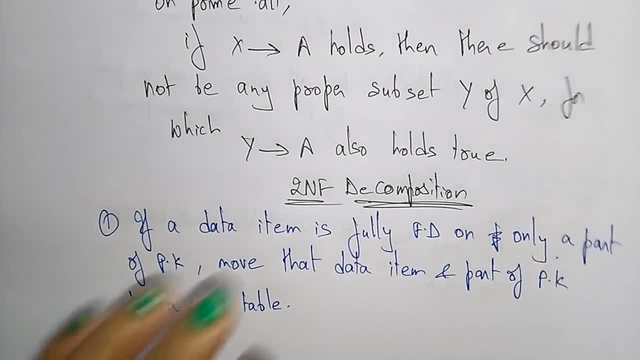 A data item that is fully functionally dependent on only a part of primary key, then you move that data- what is the data item that is there along with the part of a primary key- into a new table. Now, coming to the second step, 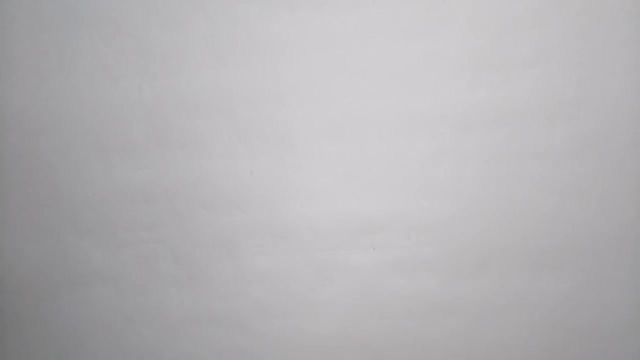 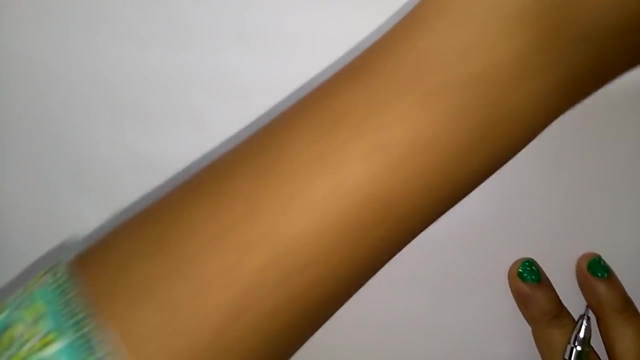 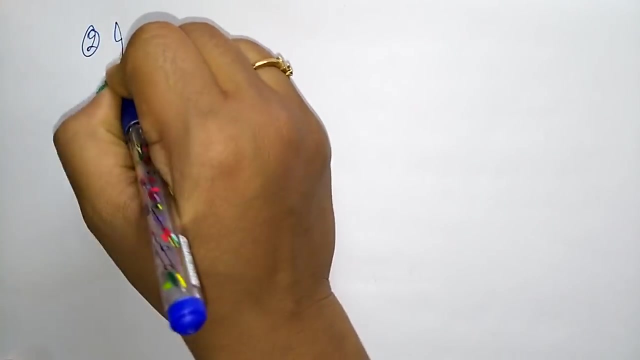 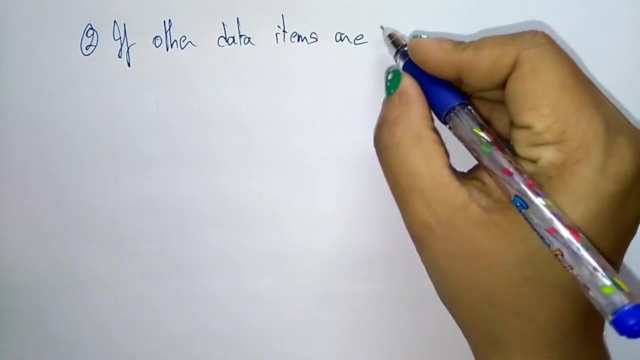 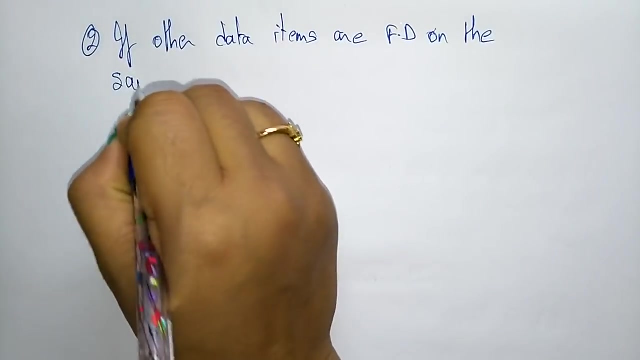 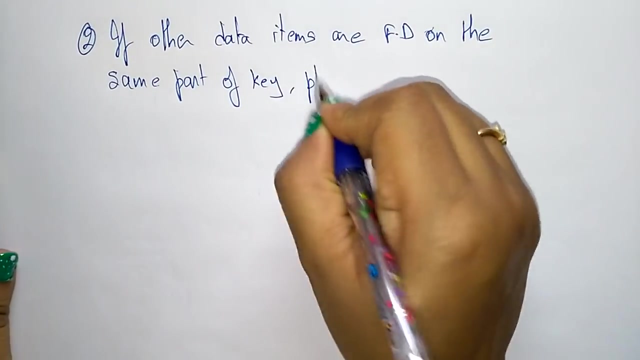 what is the second step you have to follow for the decomposition. So the second step is: If other data item or functional dependent on the same part of key, then place them in a new table. Place them in new table. 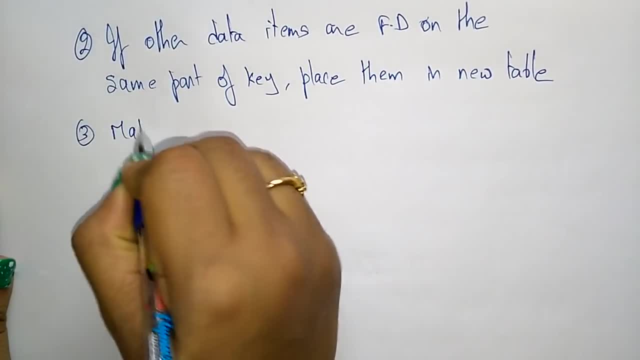 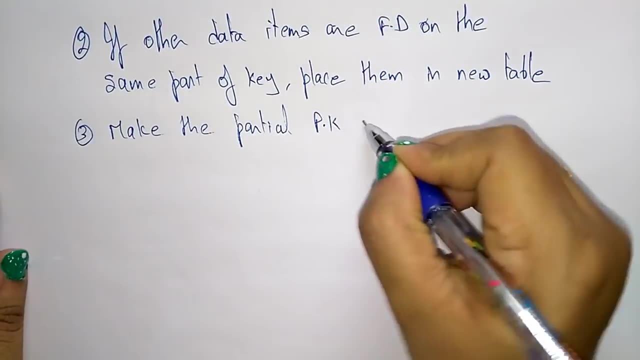 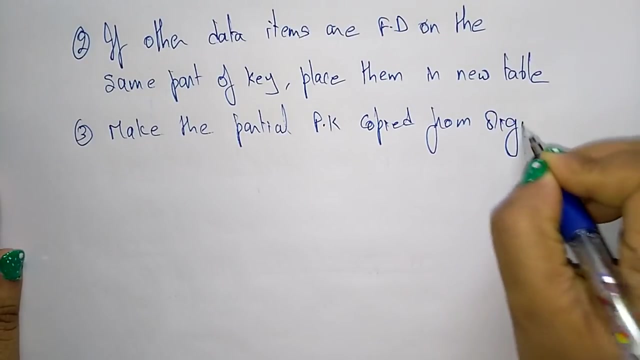 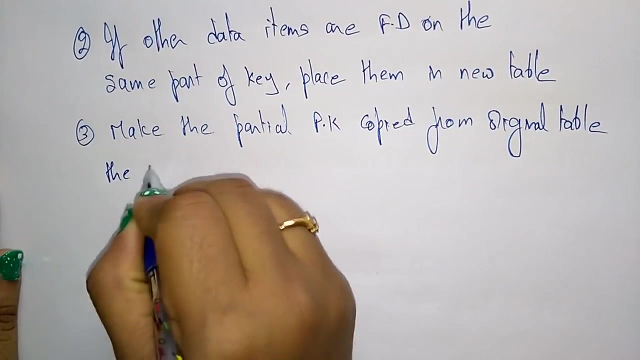 So third step: make the partial primary key not fully dependent, partially primary key copied from original table. So which is copied from original table, the primary key, then make it as the primary key for new table. 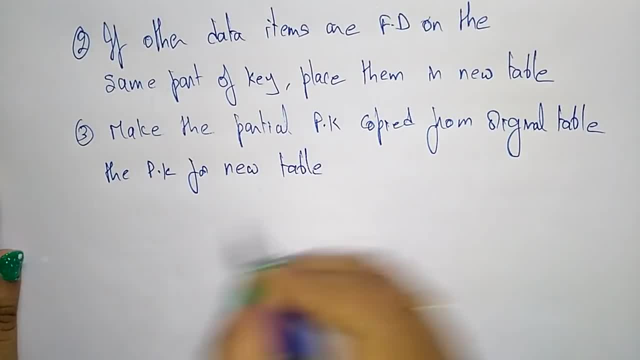 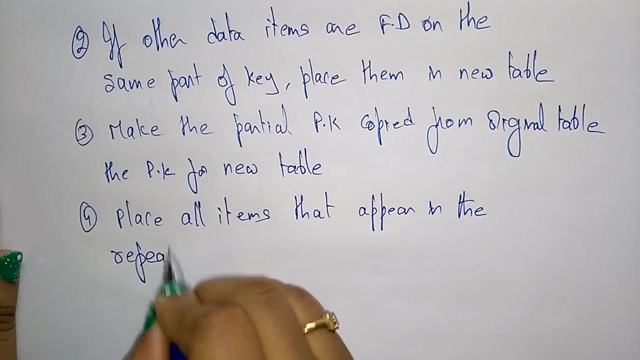 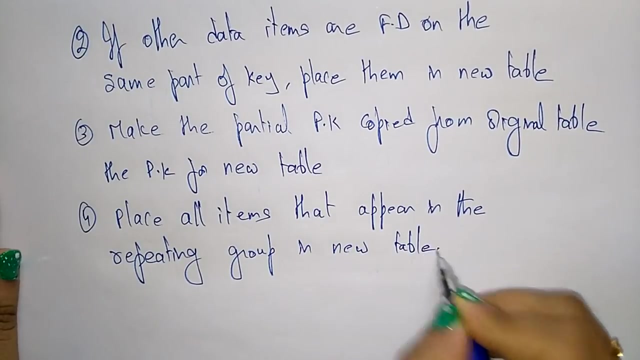 And next place all items that appear in the repeating groups in new table. So these are the steps you have to follow if you want to decompose the table into 2NF. So let's see the example for this. 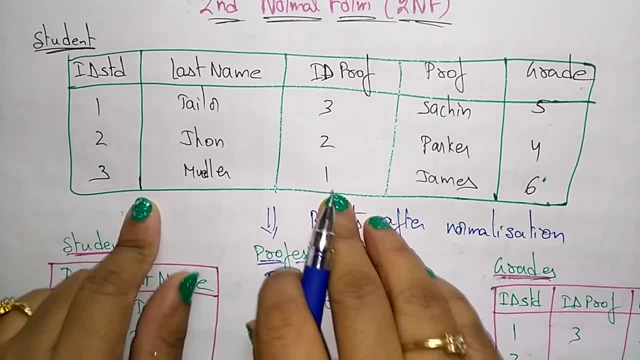 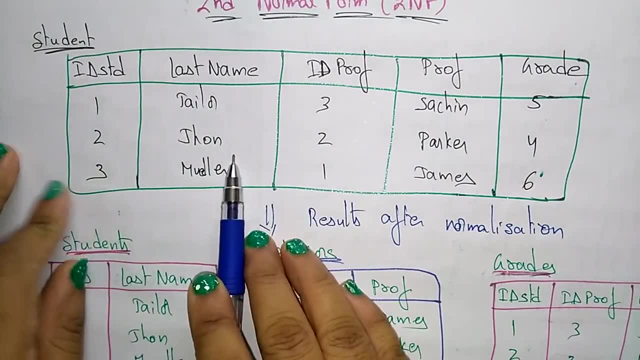 2NF, second normal form. So here I have taken a table which is not normalized having the redundant data. So here the student ID is 123, and the names of that student and ID professor- a professor ID is there. 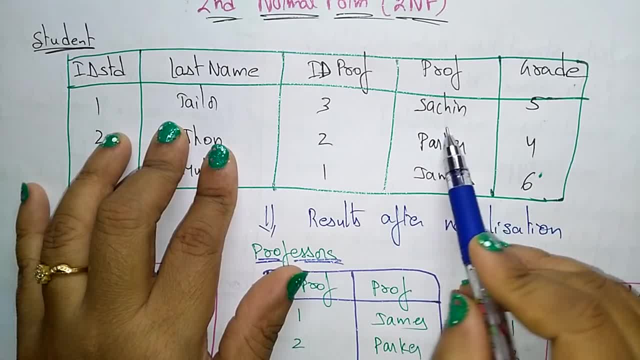 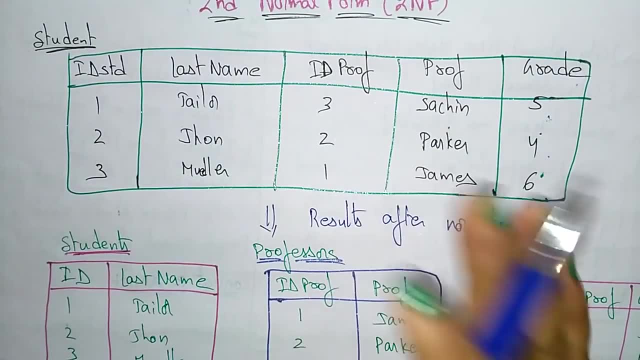 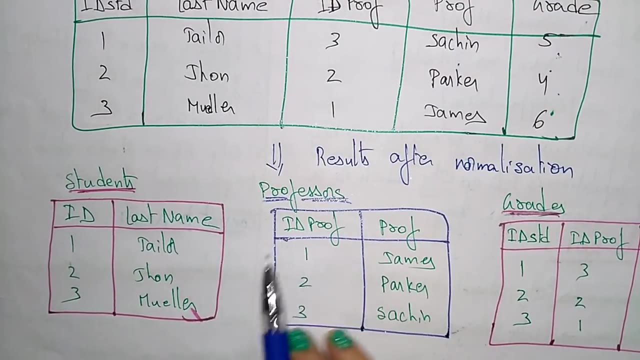 and a professor related to that student is professor name and their grades. they are relating. So this is a table which contains inconsistent data, means it is not clear. So I decompose this table into normalization. So result after normalization: 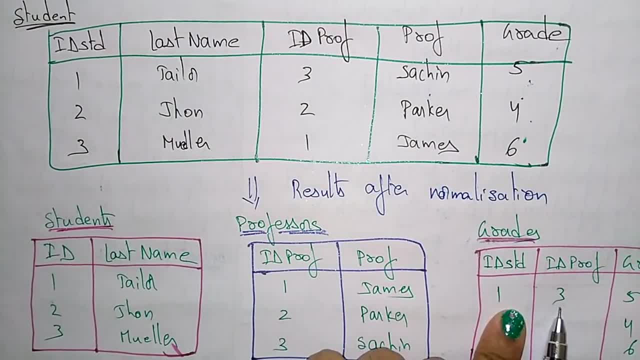 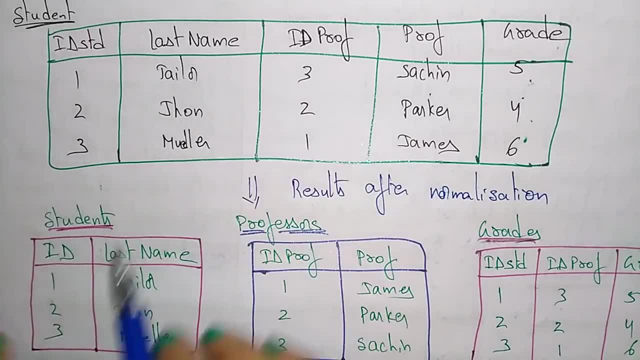 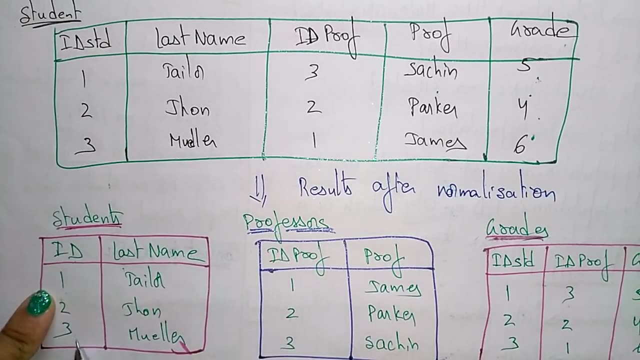 So I divide, I decompose this table into three tables, So which is having a consistent data relating to that table, So related to that table. So first I have taken the student name student table, a student table consisting of ID. 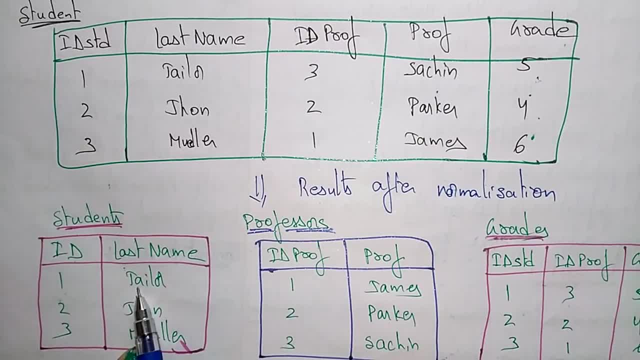 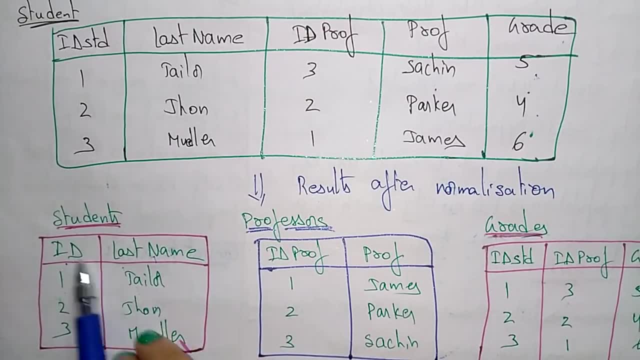 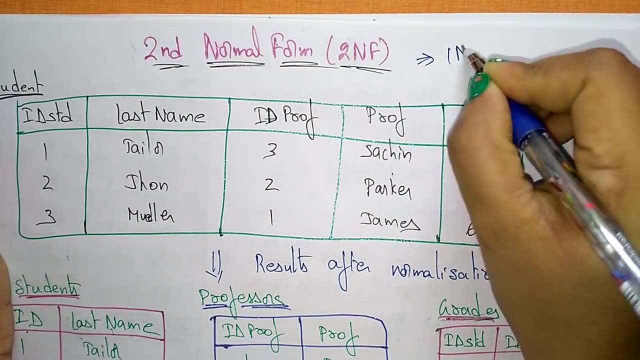 and the last name, So 123, and last name As well, as here the last name is. depends upon the ID, Means a dependency relationship. is there functional dependent relationship there? So 2NF is nothing but it has, should be in 1NF. 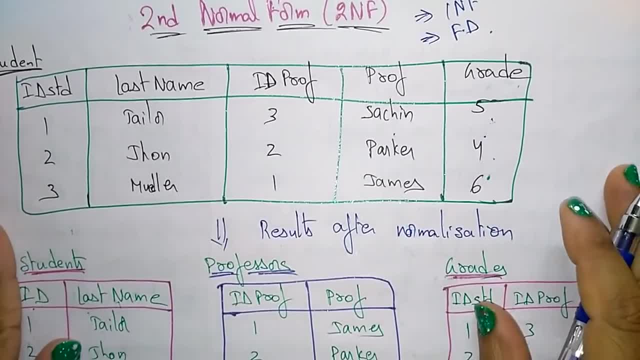 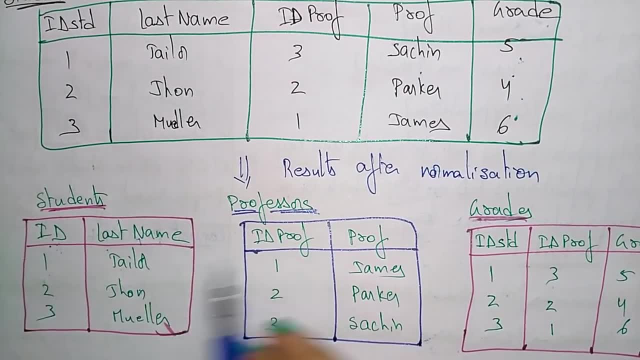 and also it exists a functional dependency relationship. So last name is dependent on ID. So last name is dependent on ID Means ID determines the last name, In the same way ID professor determines the professor. So with the help of the ID, 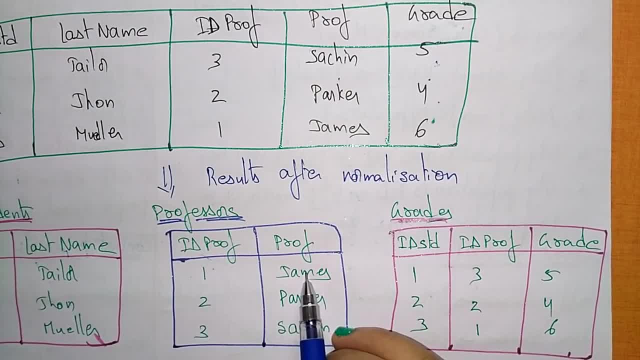 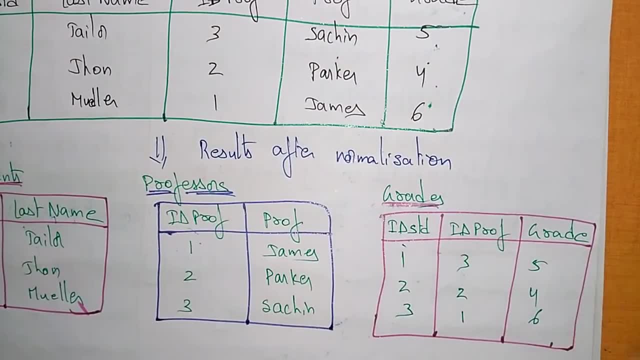 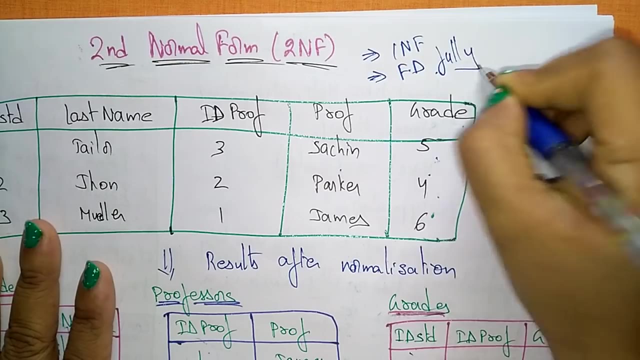 of a professor, it can determine who is the professor and who is his name. And coming to grades, So in the grades, why I am saying this 2NF, it should be fully functionally dependent. I said fully functionally dependent. 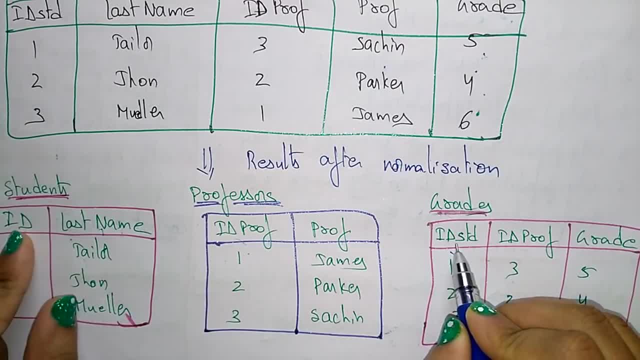 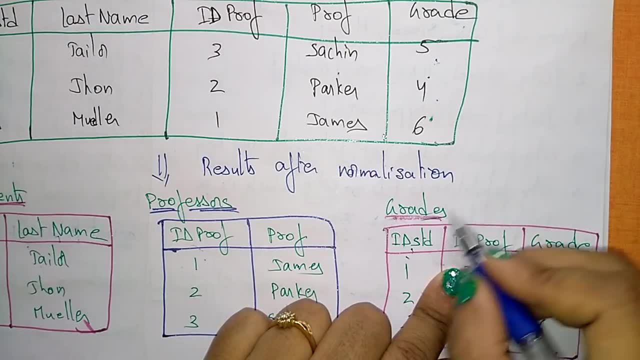 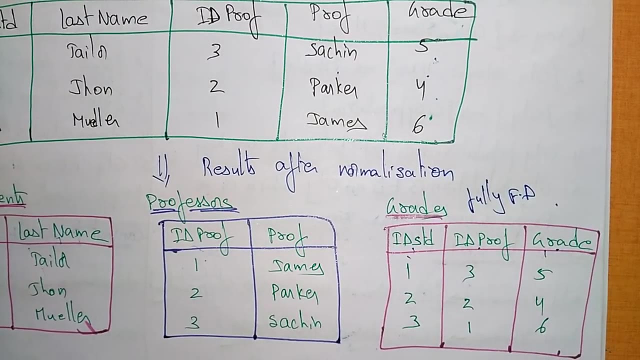 So why it is fully functionally dependent Here the ID student and ID professor and the grade. So a non-key attribute is depend upon the two or more keys. then you can say it is a fully functional dependent. So this: 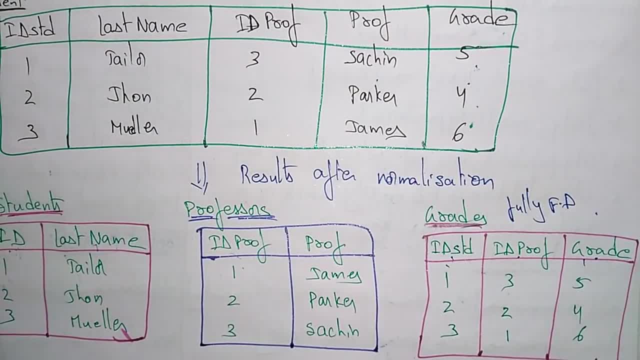 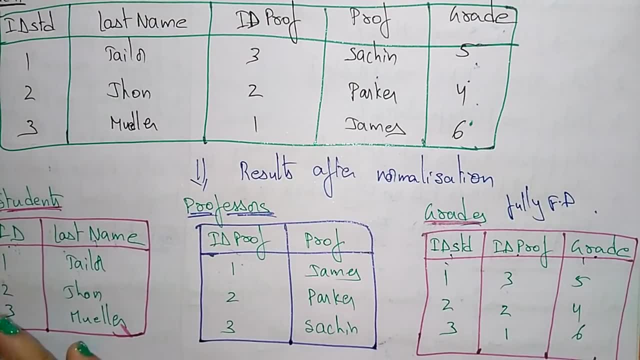 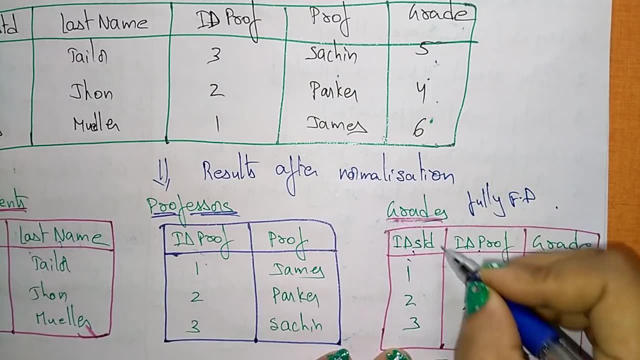 now these tables are in 2NF. So how I am saying these tables are 2NF? Because here one attribute depends upon the other attributes. Means it is following the functional dependency as well as the fully functional dependent Means one attribute depends on the. 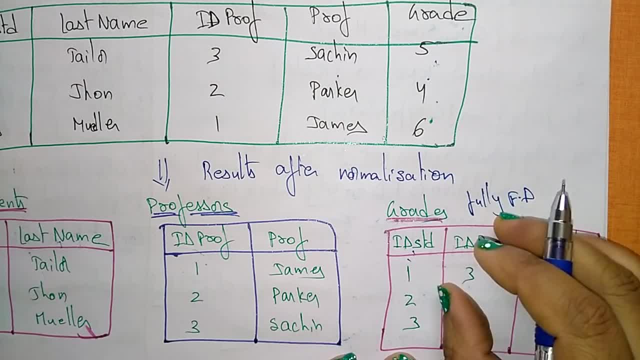 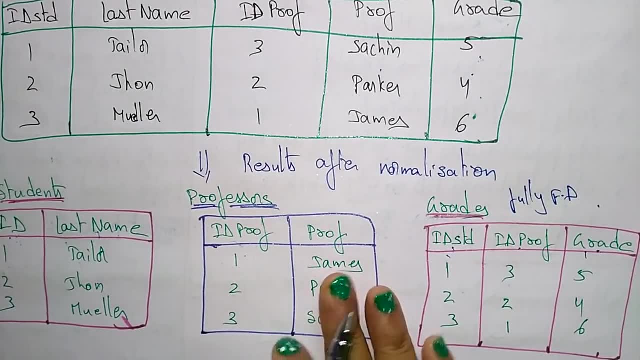 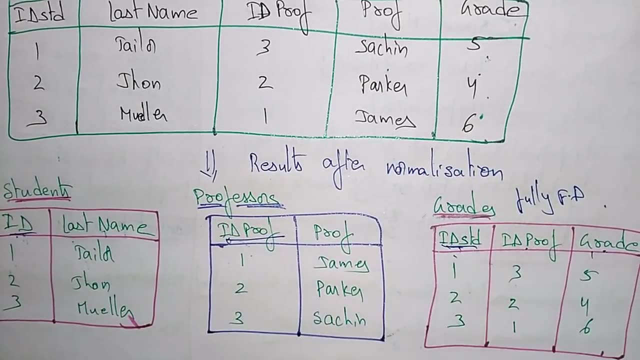 two or more key attributes, Then it is a fully functional dependent And the same way these three tables are in 1NF also Means no multi values are there And each table is having at least one primary key. Each table is having at least 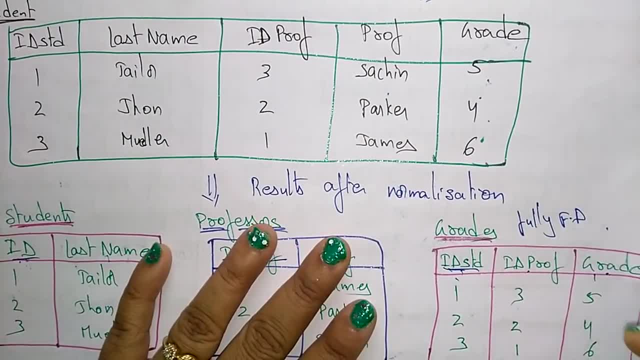 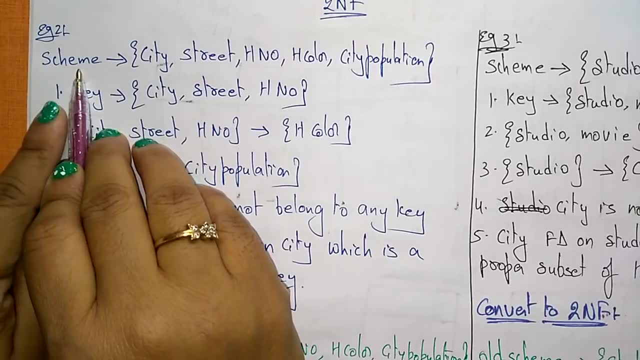 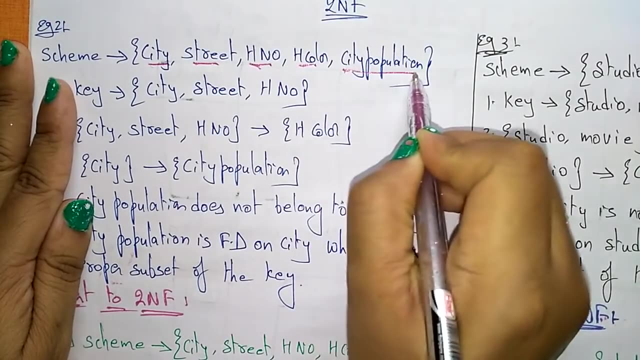 one primary key, Then you can say: this is in 2NF. So let me take another example. So here I am taking. this is a schema scheme means it is a relation table, A table consisting of attributes, house number, house color, city, population. 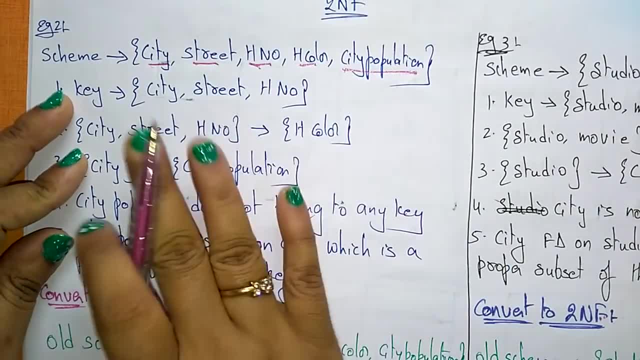 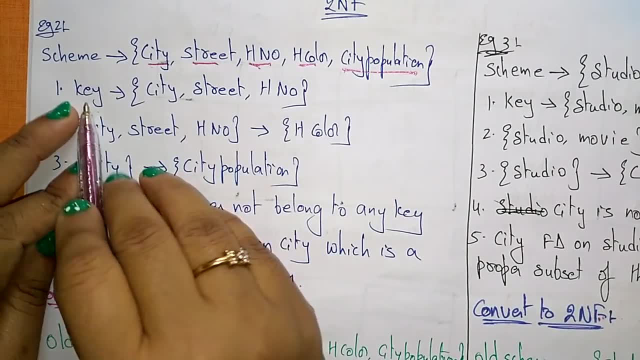 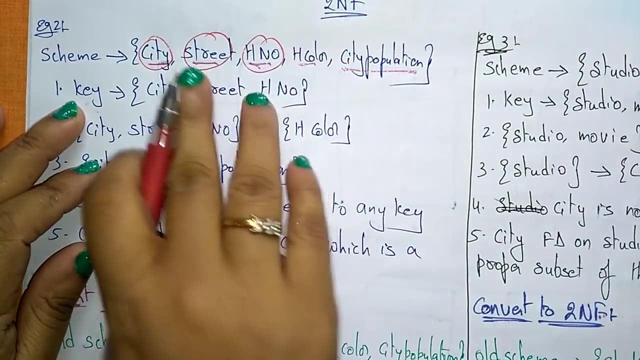 So this: now I am making this table as not in normal form, Okay, not non-normalization. So the keys in this table are. so the keys are. let us take city, street and house numbers. These three are the keys. 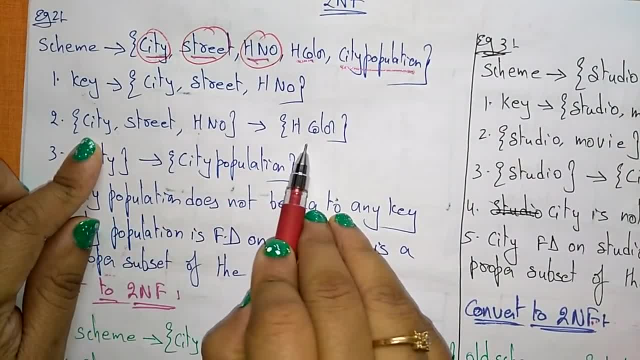 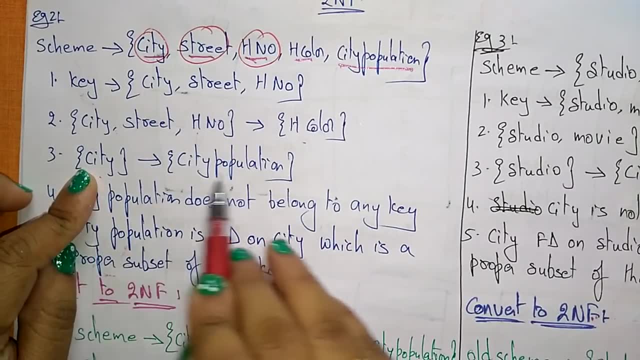 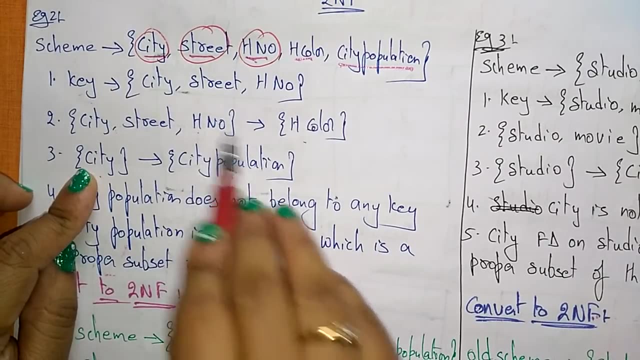 Now these three keys. all keys determines the house color. All these keys will determine the house color And city determines city pollution. population Means, house color depends on these three keys. At the same time, city pollution depends upon city. 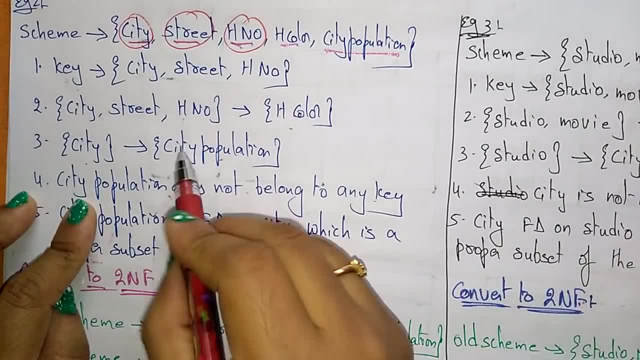 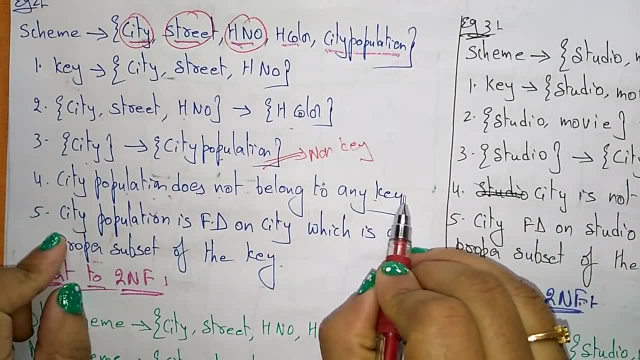 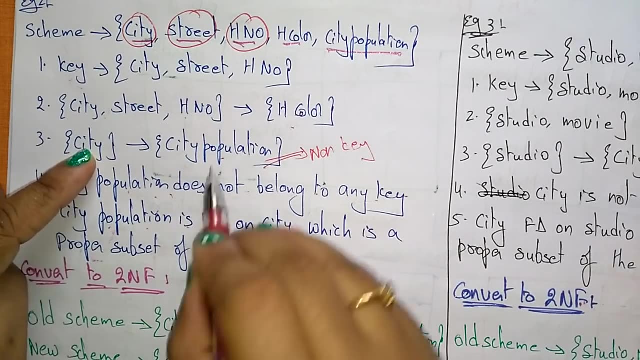 Okay, so city population does not belong to any key, So this is a non-key attribute. City population does not belong to any key, So city population is functionally dependent on city. Okay, so this is functionally dependent on city. 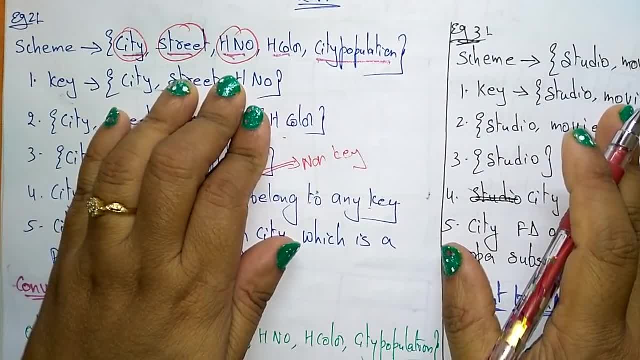 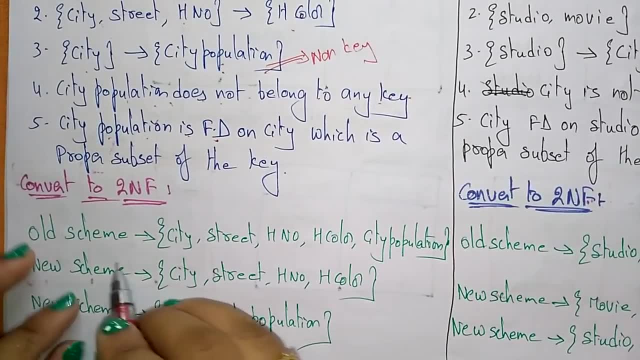 So this is a subset of the key. Now I am going to make this table as 2NF. So 2NF means it has to follow 1NF. At the same time, it should be fully functionally dependent. So this is a old schema. 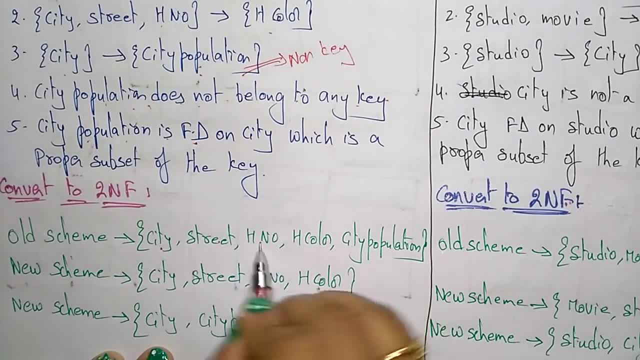 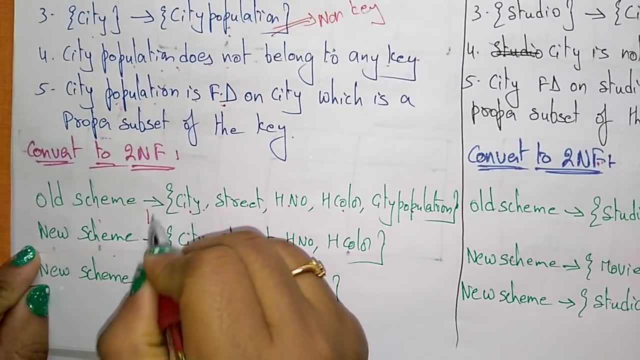 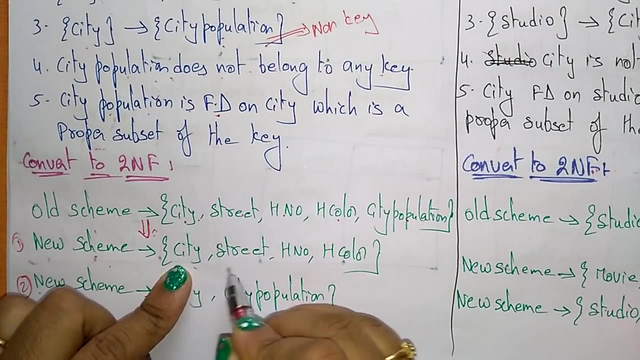 A old schema consisting of the attributes city, street, house number, house color, city population, Just this table. Now coming to new schema Means I am dividing this, decomposing this table into two tables. Two tables So, the first table consisting of street. 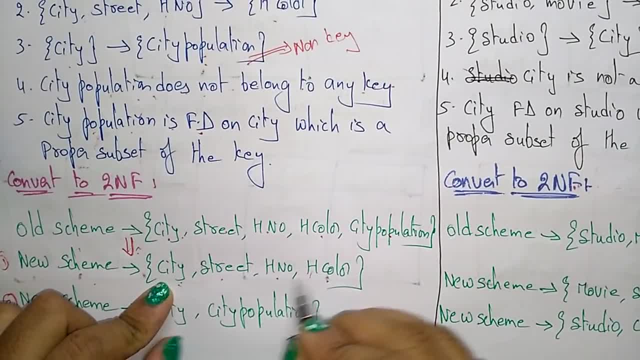 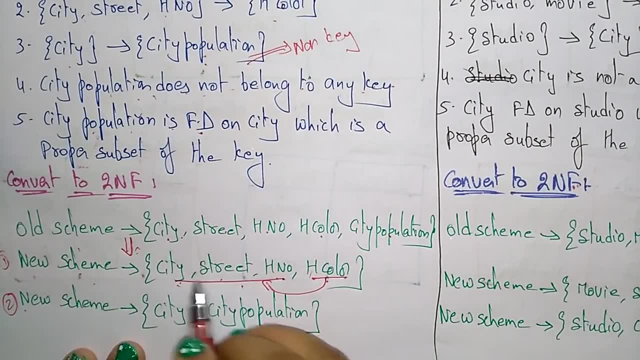 city, street, house number, house color. So this, these three are the key attributes And this is a non-key attribute. So this is functionally dependent on these three keys. So this is fully functionally dependent. Means a part of non. 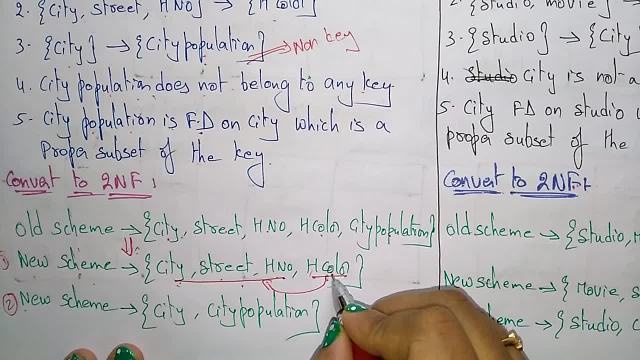 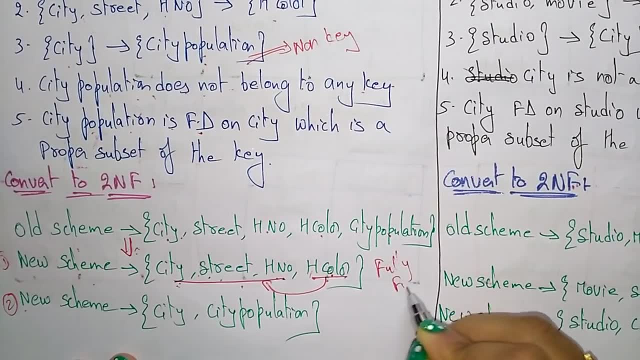 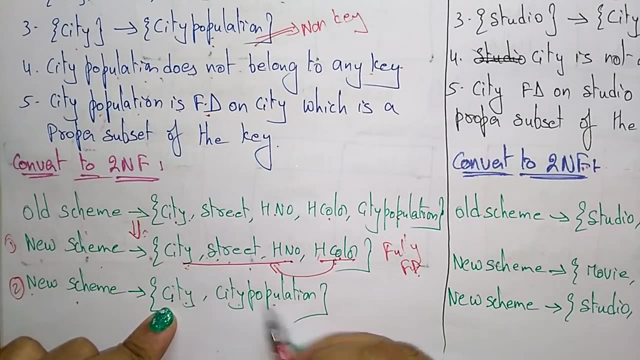 non prime attribute is depends upon the prime attributes, So this is fully functional dependent And the same way. new scheme is another table, The city comma, city population, Because city population is a non-key attribute And this non-key attribute depends upon the. 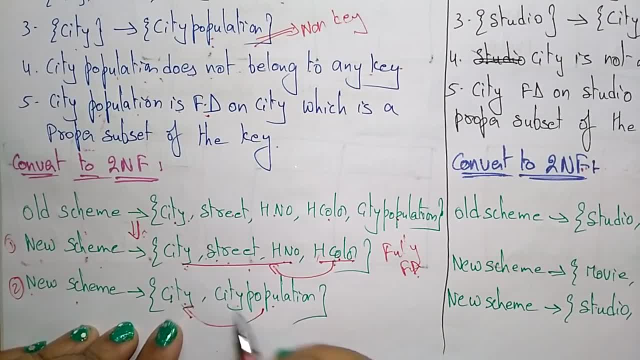 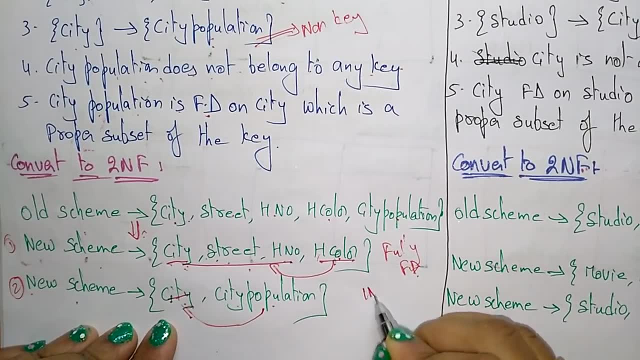 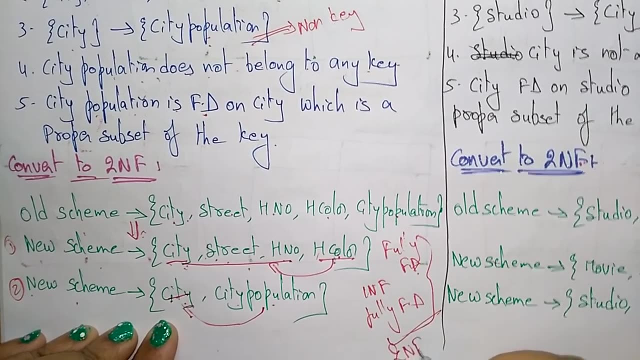 city. Okay, So here these tables are in 1NF Because each table is having one primary key- 1NF- And fully functional dependent. So then you can say this is in 2NF. So let's see, this is another example. 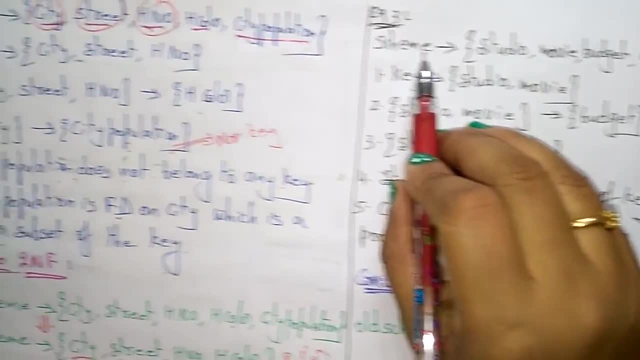 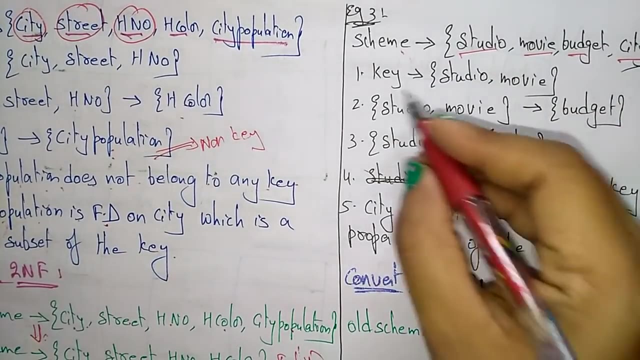 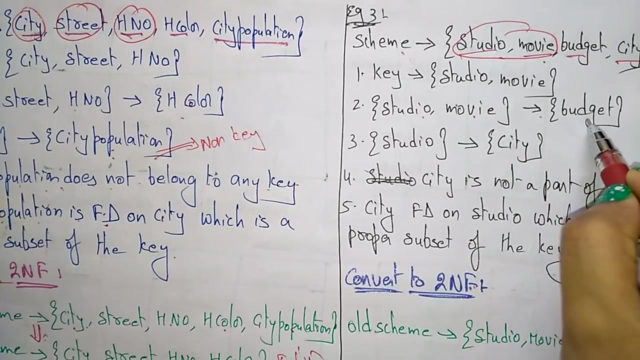 So the same. I have taken Scheme, the table consisting of the attributes studio movie budget and studio city And the keys here is: these two are the keys: Studio and movie are the keys. So these two keys determines the budget.